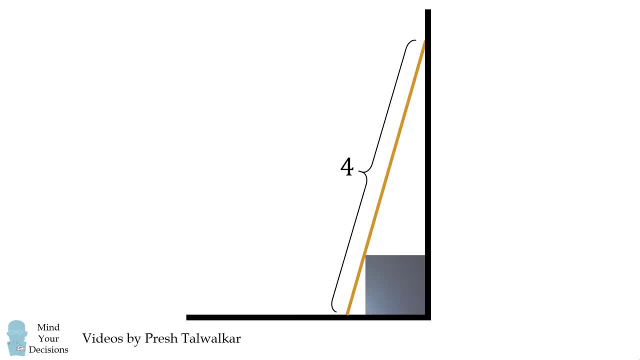 If the ladder has a length equal to 4 and the cube has a side length equal to 1,, what is the distance between the top of the cube and the top of the ladder, denoted by the variable y in the following diagram? I thank Nathaniel M, Mark L and Per T for the suggestion. 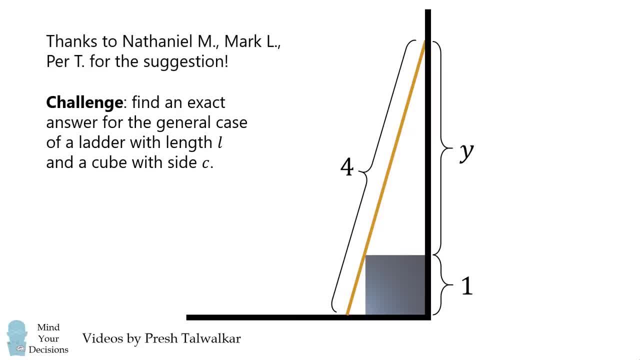 For a challenge: find an exact answer for the general case where the ladder has a length L and the cube has a side length C. Pause the video if you'd like to give this problem a try and, when you're ready, keep watching to learn how to solve this problem. 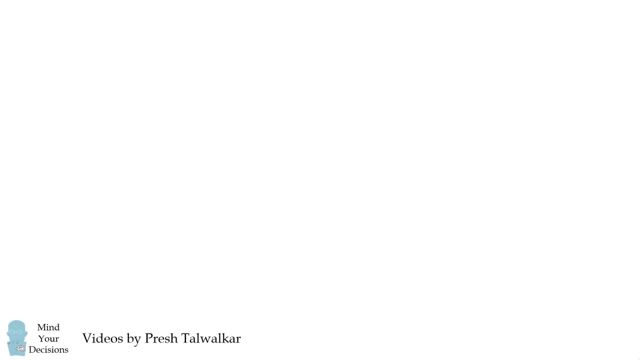 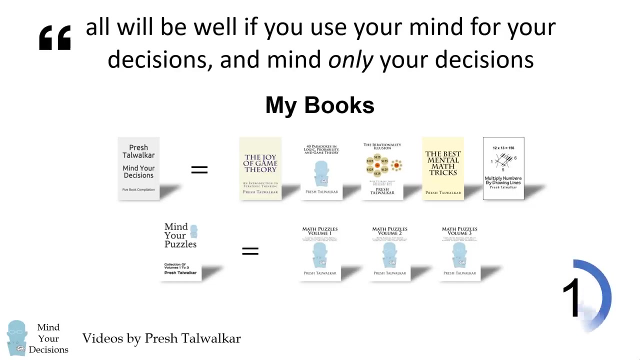 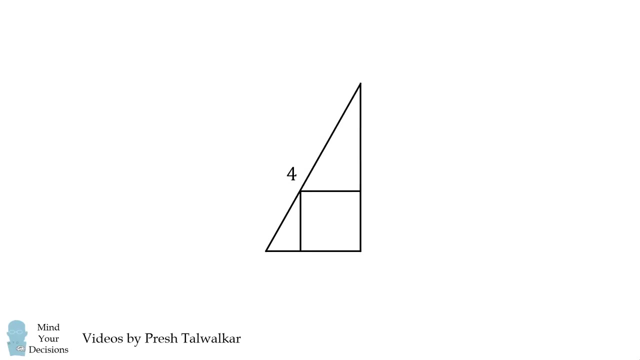 So how can we solve this problem? We have a ladder with a length of 4, a cube with a side length equal to 1, and we want to solve for the distance y. It seems simple, but it's quite complicated. 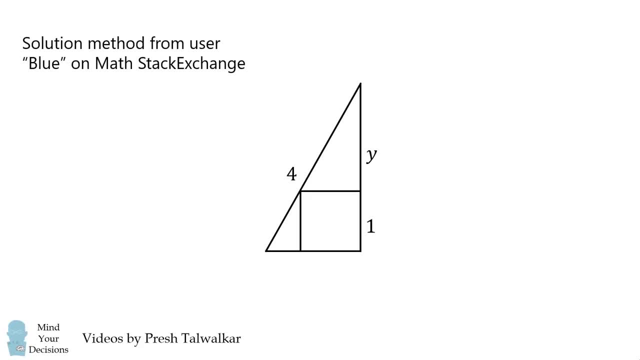 The solution I'm going to present is from the user manual. This is the answer blue, on Math Stack Exchange. I thought it was a very elegant solution. We'll get started with the general case. Suppose the ladder has a length of L and the cube has a side length C. 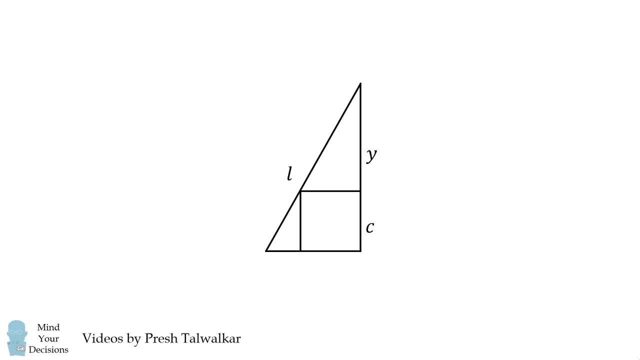 We want to solve for y in terms of L and C. To do that, let's label some more parts of this diagram. The other side of the cube will also have a length of C and we'll label the horizontal distance between the ladder and the cube as x. 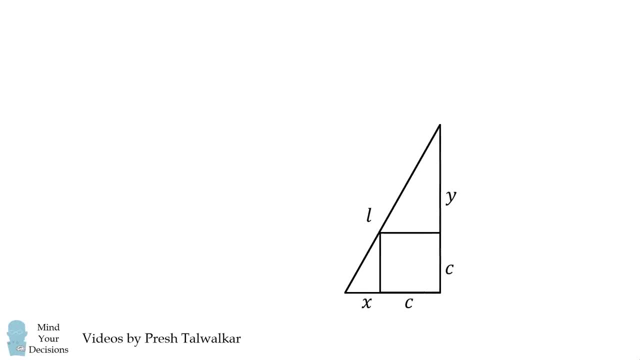 Now we're going to do a neat little trick. We're going to copy this diagram three different times and construct a square. This is going to create a clever geometric solution. We're now going to put this diagram to the side. Let's connect the four corners of these internal squares, creating another square. 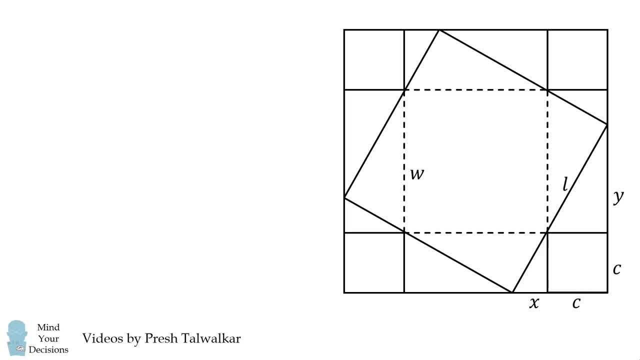 Suppose this square has a side length equal to w. Now let's label the area of this triangle where one side length is equal to x as capital X. We'll label the other triangle with a side length y as capital Y. We'll label these parts in other parts of this diagram. 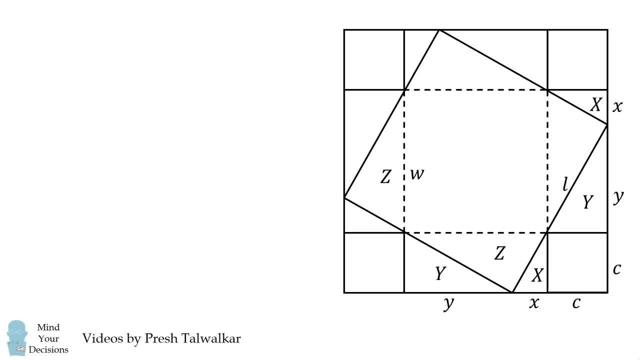 Now suppose this triangle has an area equal to z. By symmetry, these will also have areas equal to z. And just so we don't get lost, the square that consists of the four ladders we'll put in blue. Now let's calculate the area of this green square. 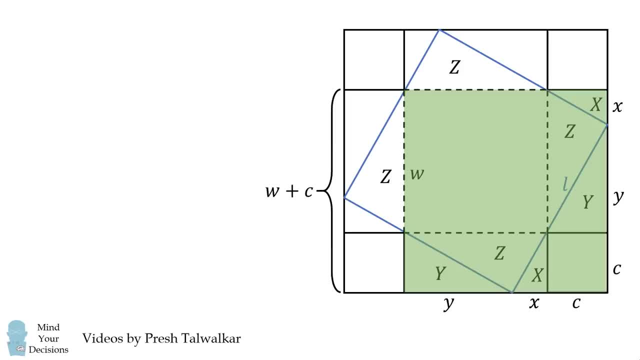 Well, one way to calculate its area is that its side length is equal to w plus c, so its area will be the quantity w plus c squared. Another way is: we'll sum up the areas of the rectangles inside of this square. Here we have a square with an area that's equal to c squared. 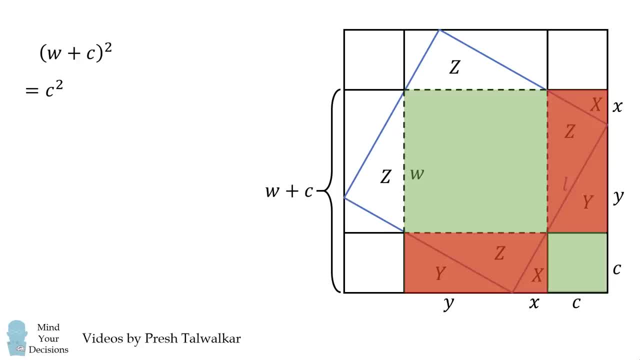 We then have two rectangles as follows: This is one rectangle and this is another rectangle. We have two x terms and two y terms, so we have two times the quantity x plus y, and we have two z terms, so we get plus two z. 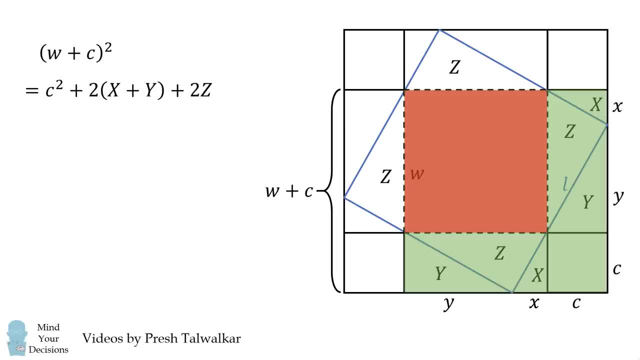 We also have this square which has a side length equal to w, so its area will be w squared. We can simplify this formula a little bit. Consider this rectangle: One half of its area will be equal to z, and one half of its area will also be equal to x plus y. 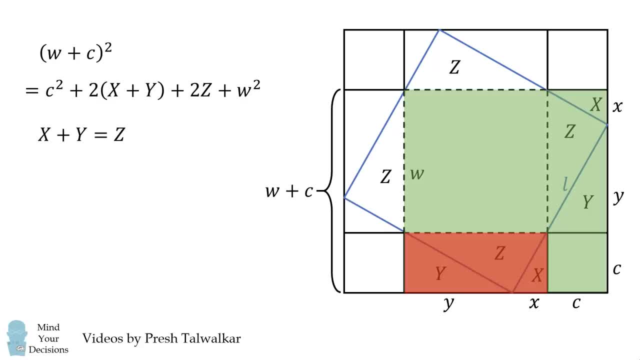 Therefore x plus y is equal to z. We substitute that in into this term, x plus y, and it will become two times z. We then group the z terms, so we have four times z. We now simplify this formula one more time. 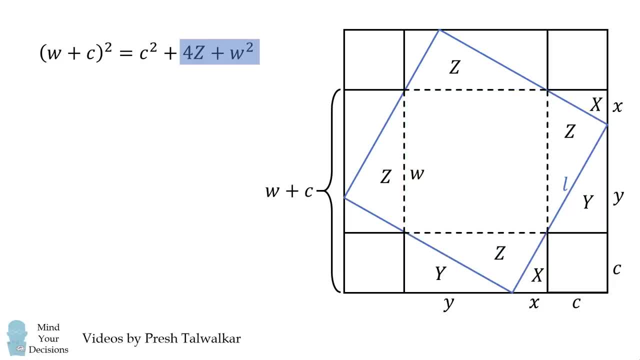 We have four z plus w squared. What's that equal to? It will exactly be equal to the area of this square which has a side length equal to l. Therefore, four z plus w squared is equal to l squared, and we substitute that in. 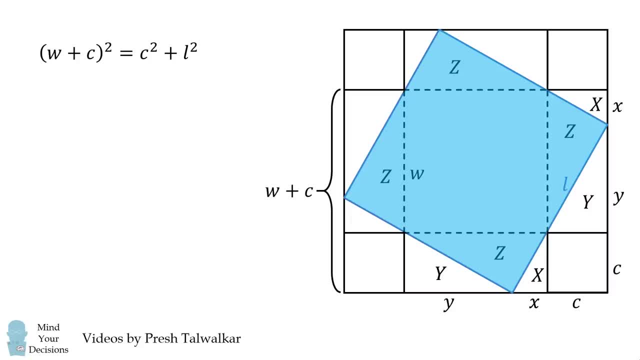 We now have a very simple formula. We take the square root of both sides, and we'll take only the positive square root because we're considering positive lengths. We then subtract c from both sides and we get an equation for w in terms of the known values of c and l. 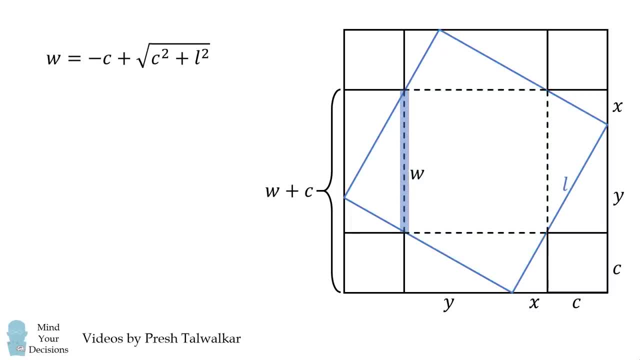 We now make one observation about w. w is exactly equal to the side length of this square, which is equal to the quantity x plus y. So we have w is equal to x plus y and we want to solve for y. To do that, we'll consider these triangles.